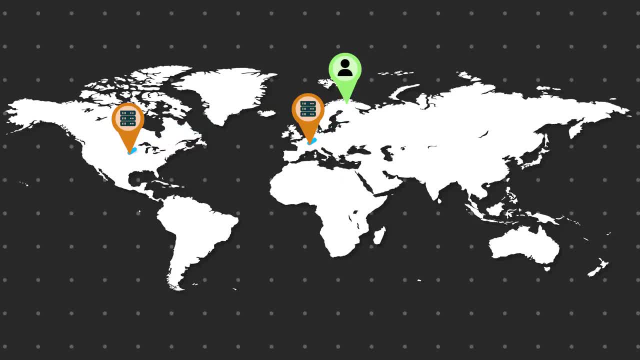 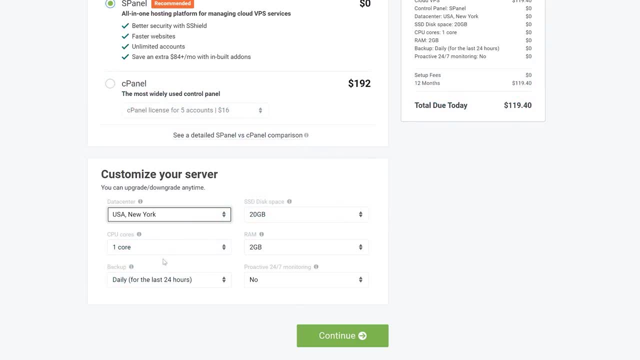 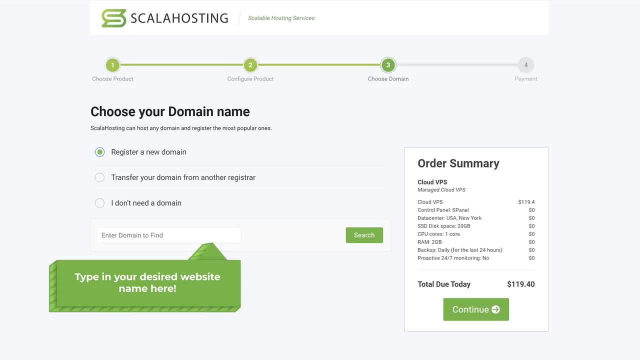 The closer they are to the user, the faster your website will load to that user. So pick this based on your target audience location, not yours. Now click continue Using Scala Hosting. you also get a website name for free, So that's just another big plus. 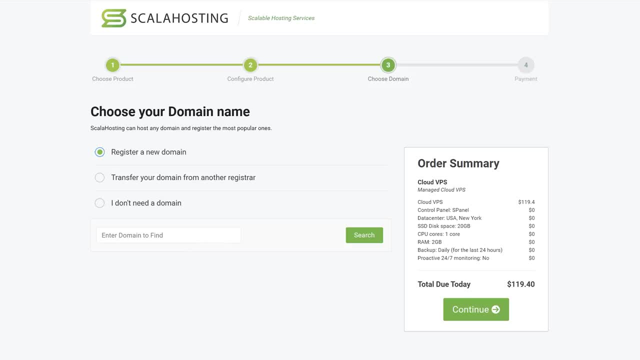 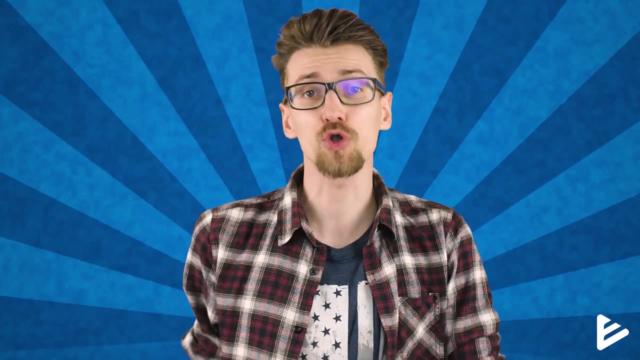 But if you already have a website name, you'll be able to connect that as well later. So just grab this free one as a bonus. Okay, so once that is out of the way, I'll show you how to set everything up, how to. 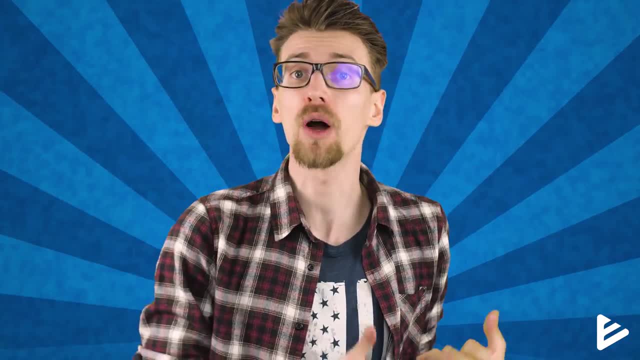 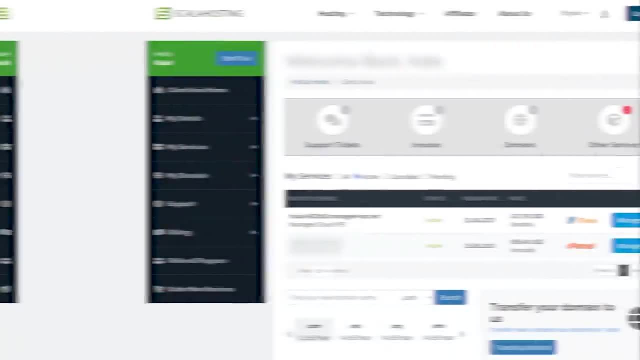 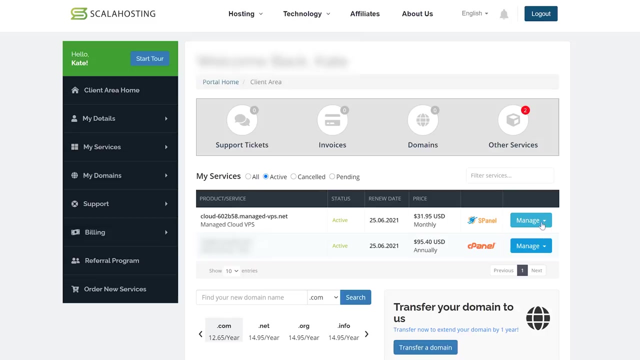 allocate resources to your server and how to actually put a website on it in the easiest way possible. Once logged in, you should see a menu like this And you should have your plan already added, So just click on manage and then manage service. 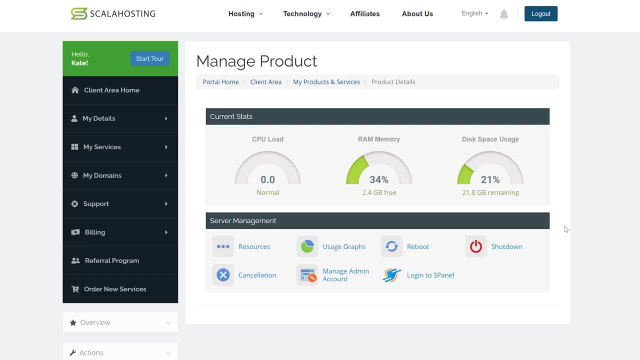 Now you're inside your server controls. You can see how many resources you're using up. You can restart your server or shut it down completely, if you like. Most importantly, if you want to add or remove resources, you can do so by clicking on the. 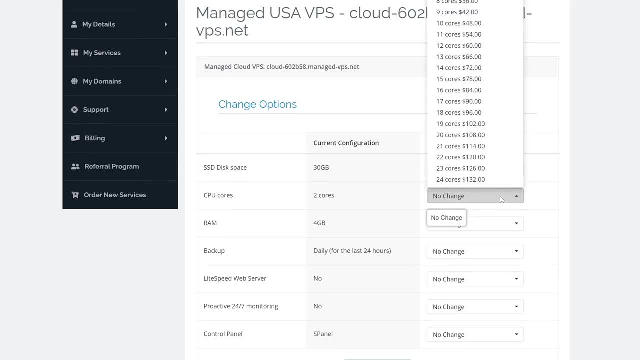 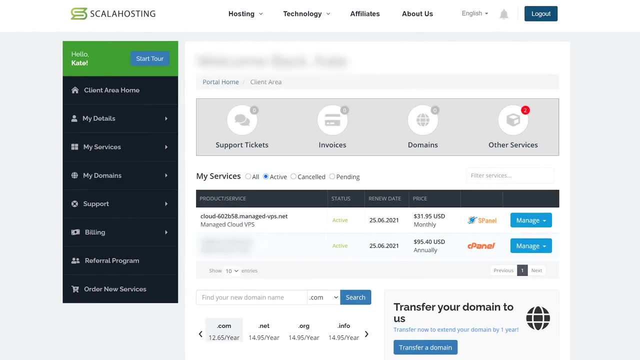 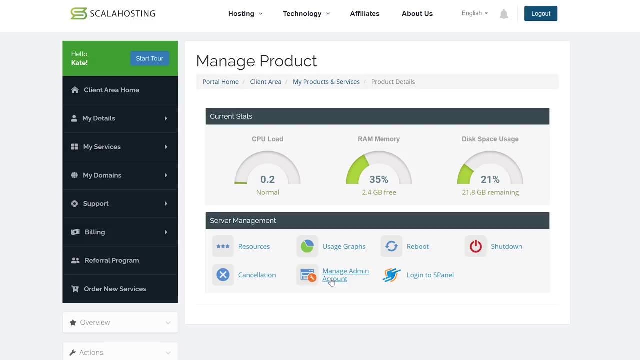 resources icon and just changing these values around. Keep in mind that extra resources cost extra money. But anyways, if we want to put a website on this server, you'll need to create an admin account for yourself first. So go ahead and click on manage admin account and create an admin account for yourself by. 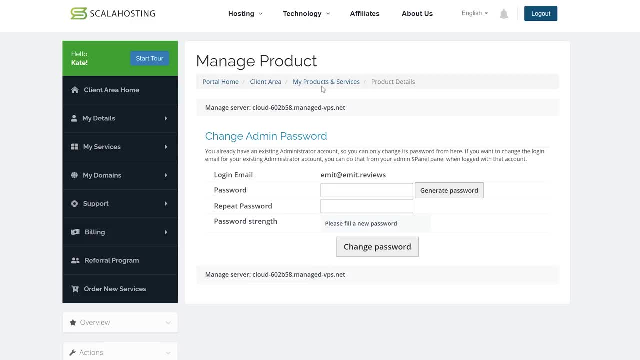 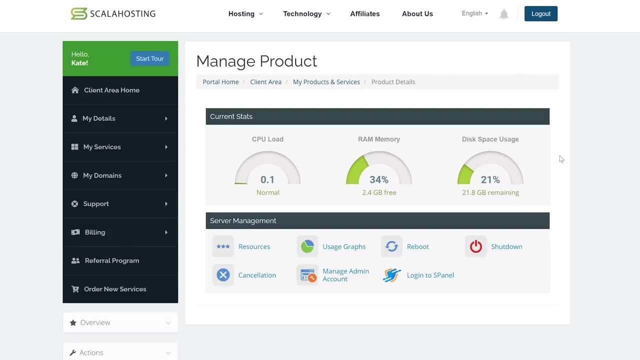 typing in the login email and password. I've already done this step earlier. Then click on my products and services at the top here. Go back to your server management area. Click on login to S panel and use the admin account you've just created. 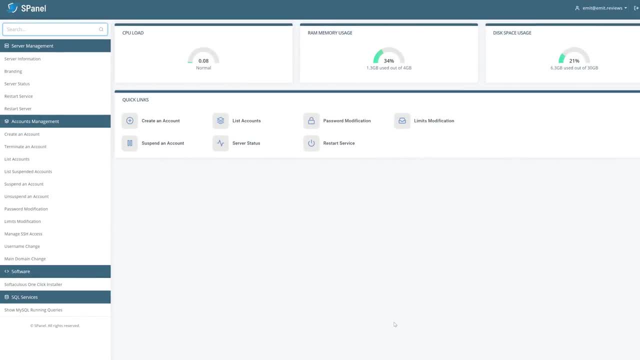 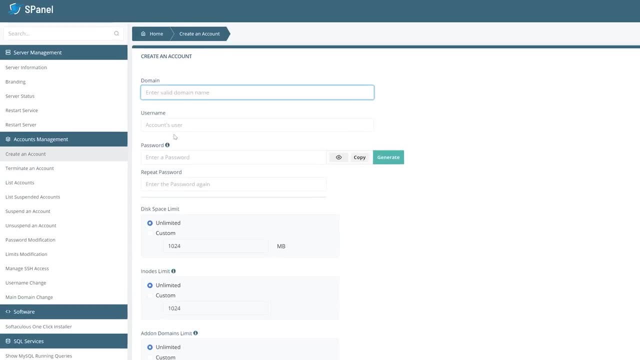 To put a WordPress website on here, you'll need to allocate resources for the website. So first things first, click on create an account Type in your website name. This can be the domain name you've got on Scala hosting, but I'll use a separate domain. 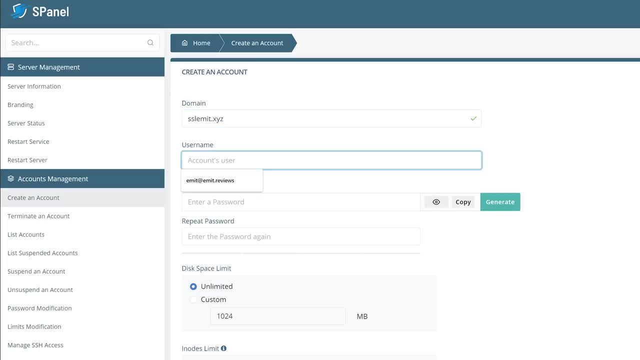 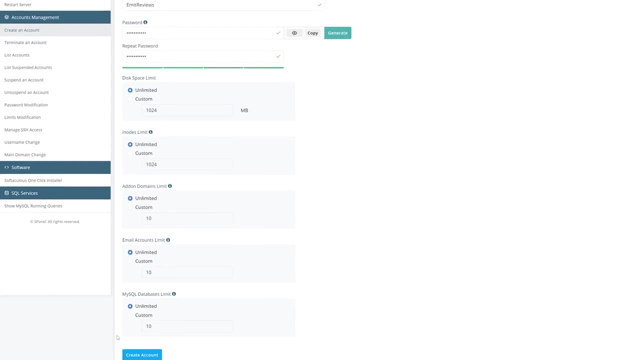 I've bought elsewhere, and I'll show you how to connect it to Scala hosting. Think of a username and password for your website, And then choose the limitations. If you're creating a website for yourself, you can keep this unlimited. If you're using this server to host a friend's project or something, you can definitely add. 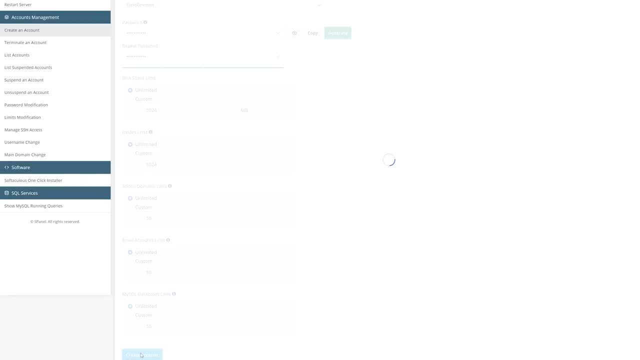 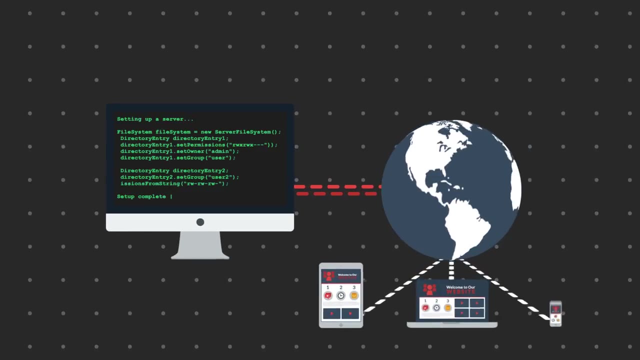 some limitations. Finally, click on create account. Now you'll get some information about your account. Since I used a domain I bought elsewhere, I'll use this information to update my name servers. so the website name points to this website I've just created. 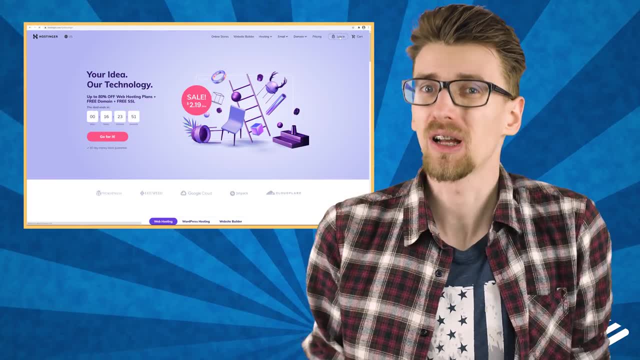 I bought my domain name on Hotspotcom. Click on create account. You'll see the domain name on Hostinger, so that's what I'll use, But the process is generally the same absolutely for any web hosting provider that you use. You just need to find the DNS or name server area and change some values around. Log into the service provider where you bought your domain name and find an area called domains or DNS- In Hostinger's case it's domains- Then choose the website name you want to attach to your server. 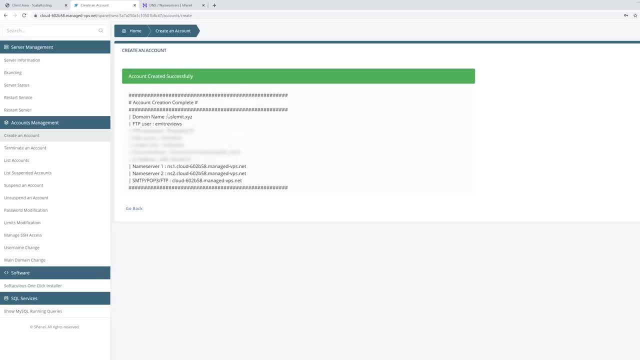 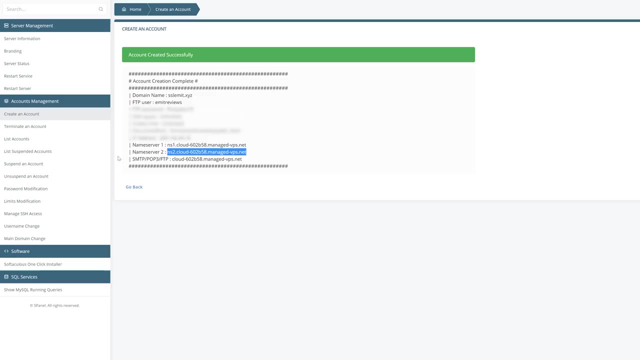 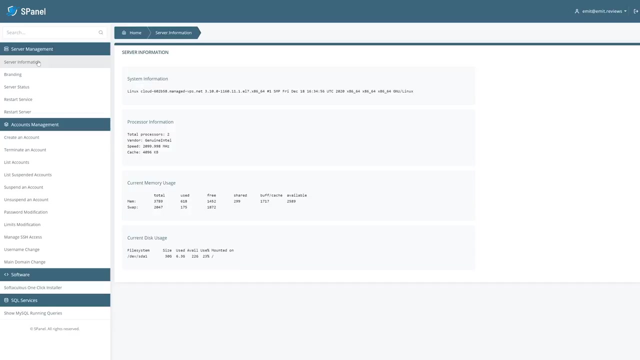 Near the name servers, click on change And type in the two names. I'm going to name servers from Scalab Hosting And then click save. If you've accidentally closed this window on Scalab Hosting, you can find the information about your name servers by clicking on server information. 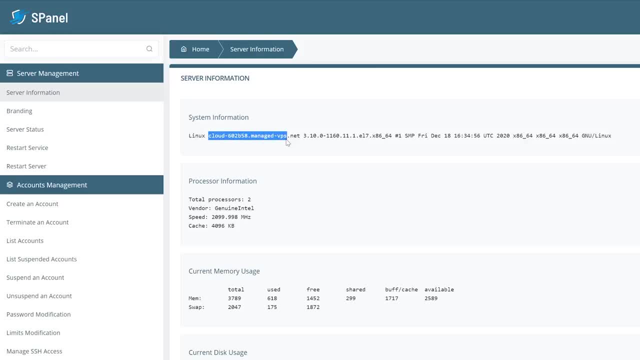 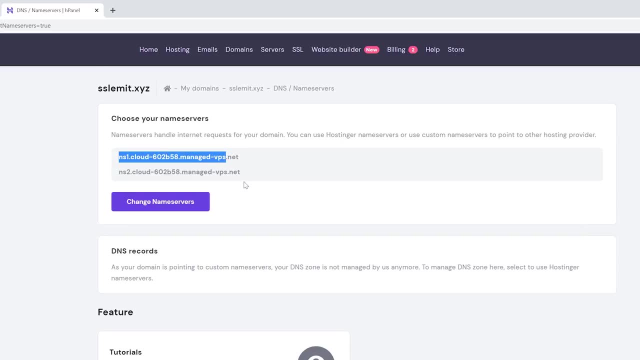 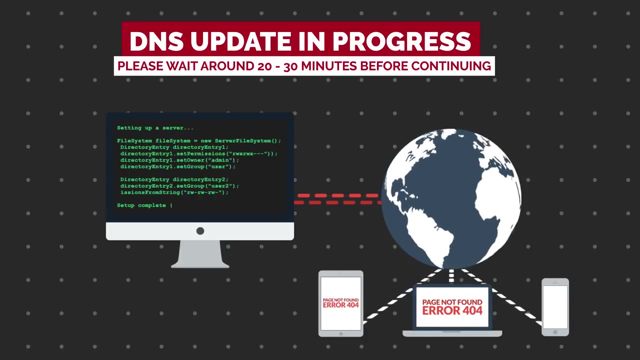 As you can see here, my name server is located here, So all I need to do is add NS1. And that's it I'm going to paste in my name servers Now. it could take up to 20 to 30 minutes before your name servers are fully updated. 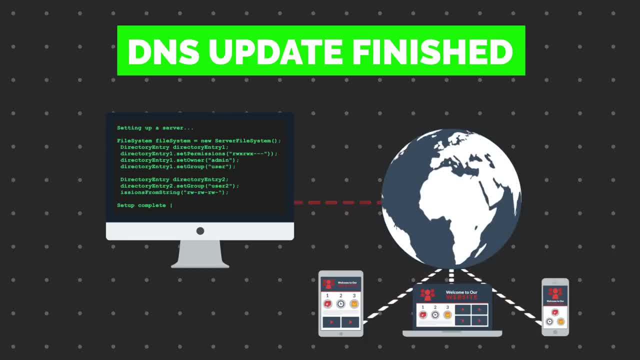 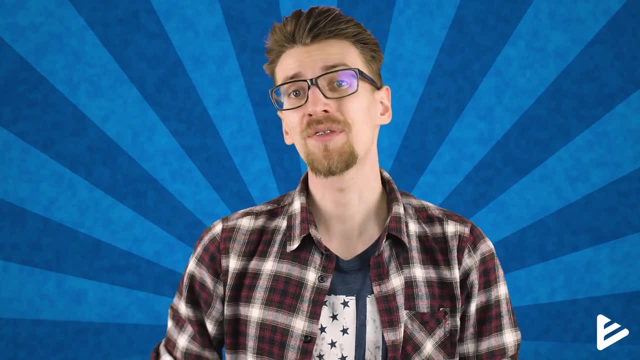 If you'll get any errors on further steps, just wait a bit, because probably the name servers haven't finished updating So far. we've bought a virtual private server, We've set it all up and allocated enough resources for our website, So the only thing that's left to do 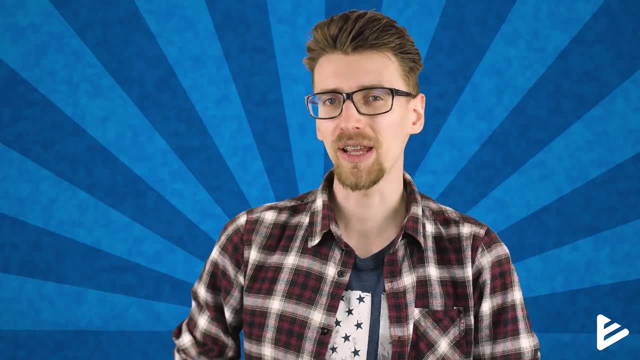 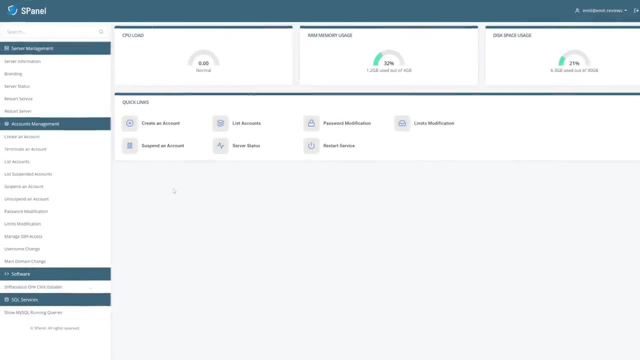 So far, we've bought a virtual private server, We've set it all up and allocated enough resources for our website, So the only thing that's left to do is actually put the website on there and enjoy a fast and secure experience. Once inside your server management panel, click on list accounts and you'll see all. 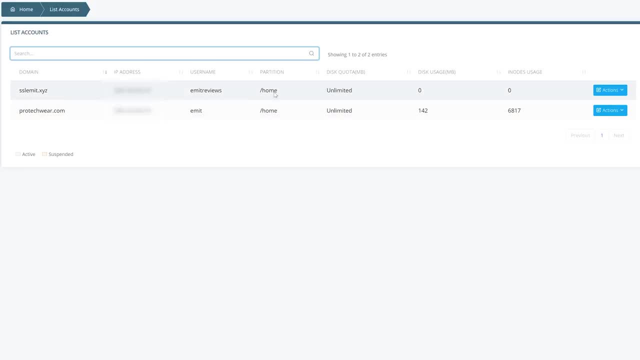 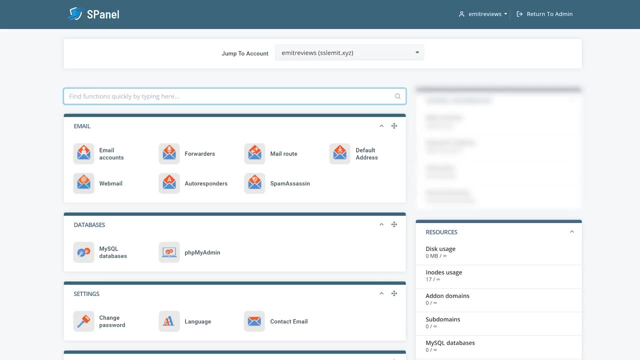 of the different websites you're hosting on your server, Click on actions and log in next to the website you want to manage. The first thing we'll do is add WordPress onto your server. Since Scalab Hosting is a managed service, it will be really easy. 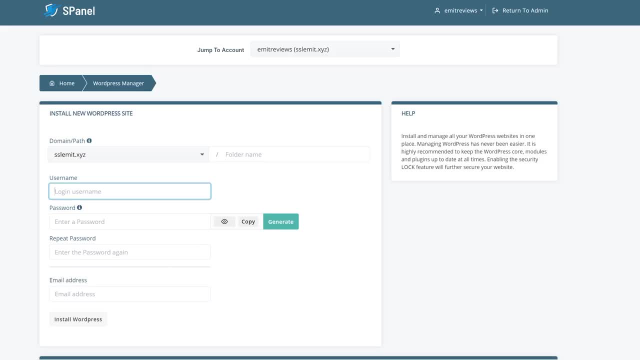 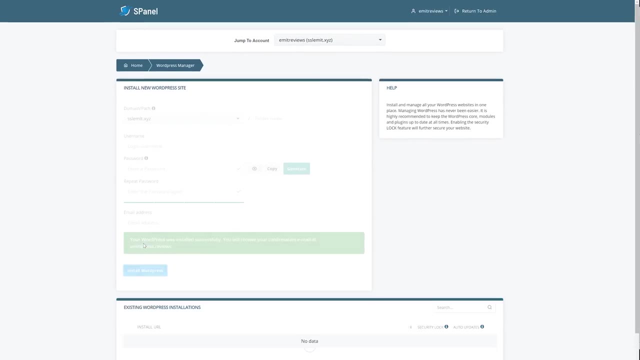 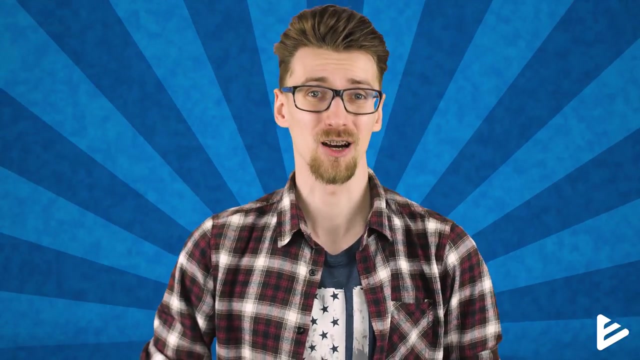 Click on WordPress manager and then think of a username and password for your WordPress dashboard, Type in an email address where you get updates and click on install WordPress. Since we're using the script that's provided by Scalab Hosting, the installation will only take a couple of minutes and everything. 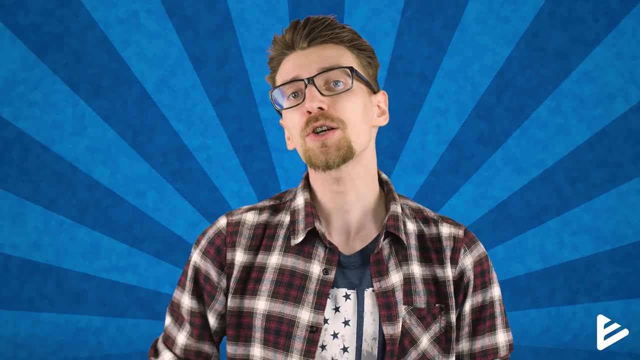 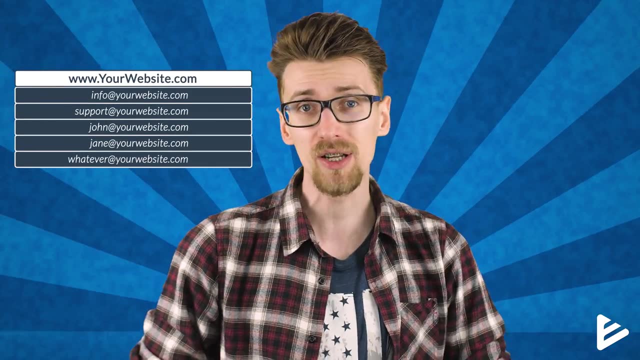 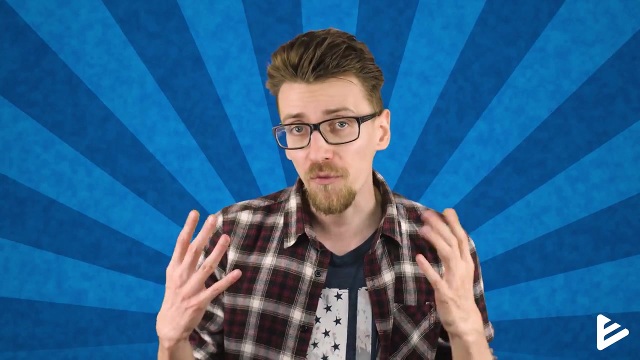 is done automatically. However, once that's done, let me show you two more very important aspects for your website. That is, how to create a professional email address using your website name and how to encrypt your website for free using an SSL certificate. Both of these things can be done using the S panel, and we're going to do them right now. 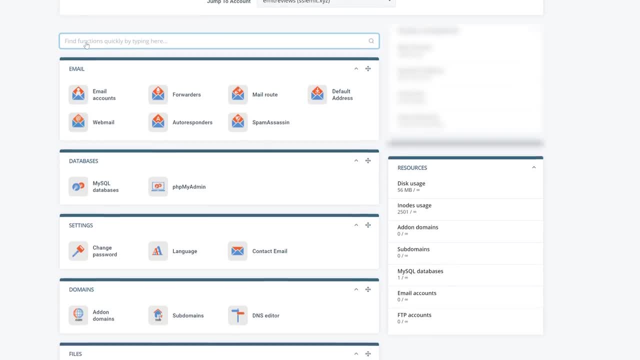 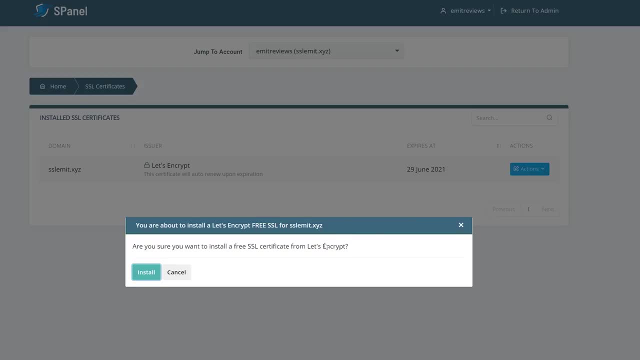 To encrypt your site, go back to your S panel and click on SSL certificates. Then click on actions and install. Once you've done that, just click on cancel. What this does is it adds a padlock next to your website name instead of a not secure tag. 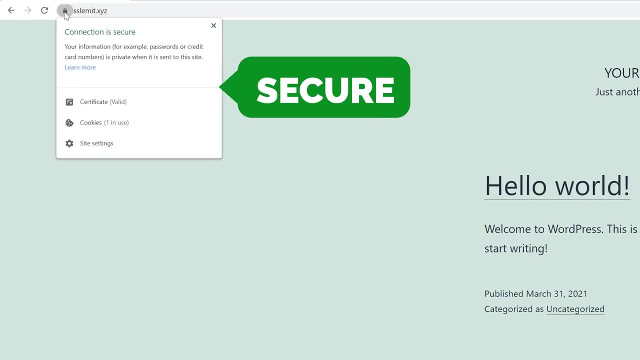 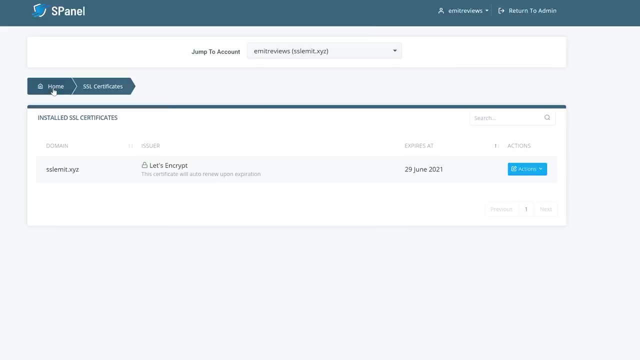 Next go back to S panel. You can click on home from the SSL screen, Then click on email accounts and create an email with your domain name. I'll do info at SSL dot XYZ. Then just think of a password Now if you want to access this email address. 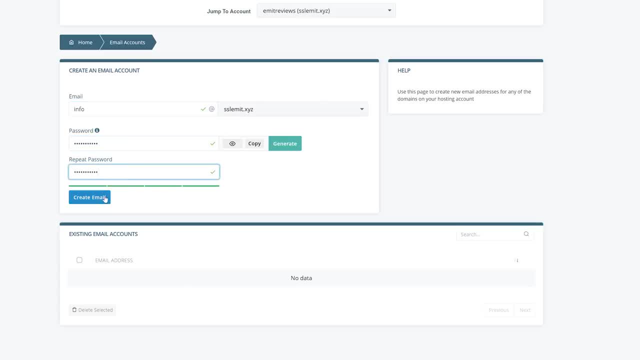 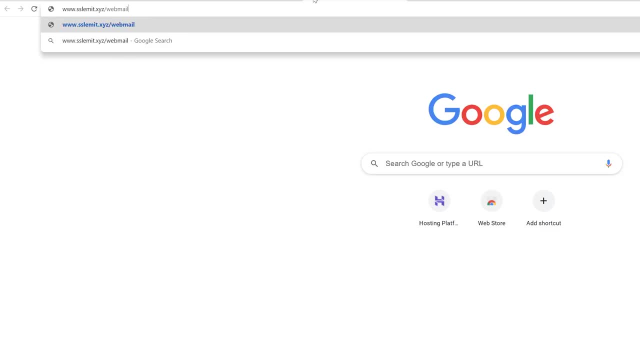 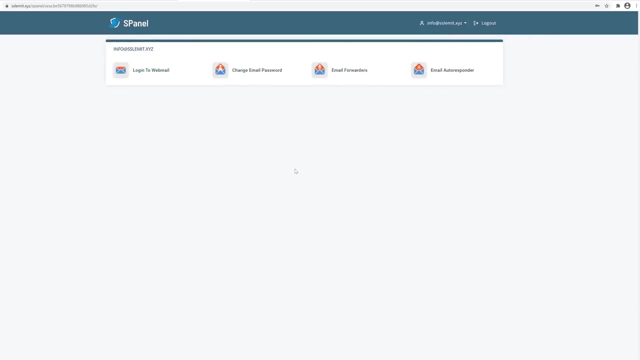 just click on the email address and then click on the email address. Then click on the email address. Just type in your website name, followed by slash webmail, and use the login information you've just created. Then click on login to webmail and you'll see all of your emails there. 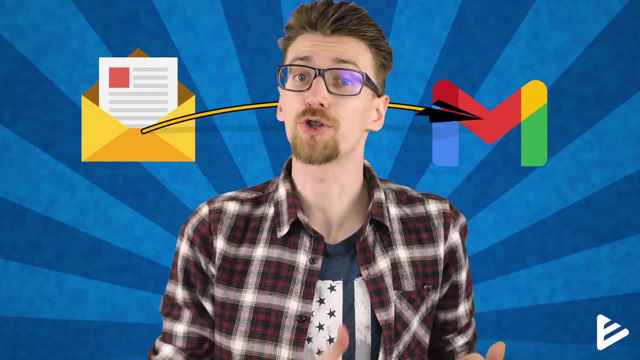 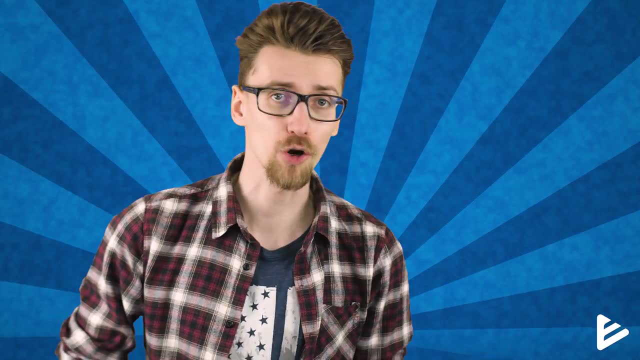 However, it is possible to link this email address together with Gmail or Outlook, So everything works faster and you just need less email boxes to navigate through. I'll leave a tutorial on how you can do that right here, my dudes, Okay, Once we have all of that, 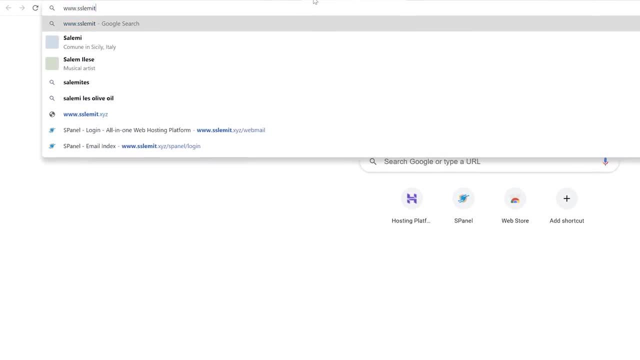 let me show you how to reach your WordPress dashboard. All you need to do is type in your website name, followed by slash WP dash admin and type in the login information you've created during the WordPress installation, And this is where you're able to manage everything in regards to your website.